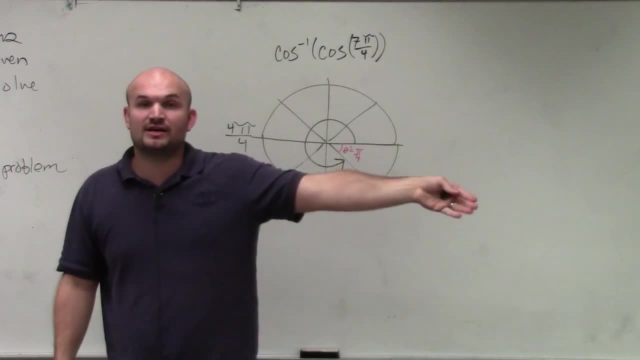 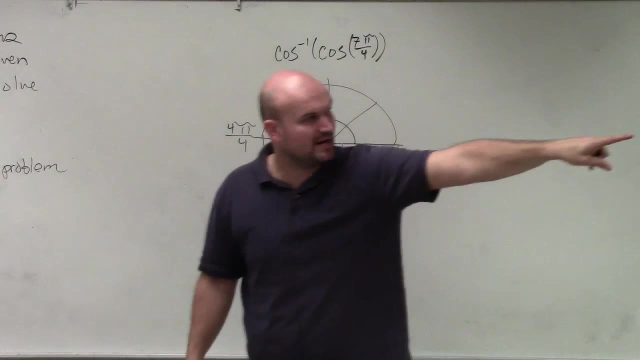 If you can always quickly find the reference angle, you can quickly find what the value is. So if we look over there and we say, oh okay, what is the cosine of pi over 4?? So we find the little right triangle that corresponds to the pi over 4, or 45 degrees. 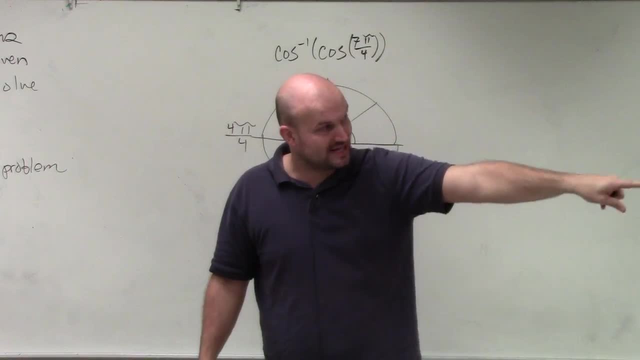 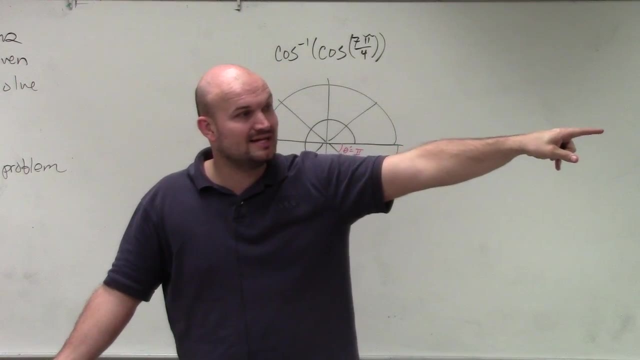 and we know that the cosine we could easily do for cosine we could do adjacent over hypotenuse or, since we're looking at the point on the unit circle, we could just use the x-coordinate. So the cosine of pi over 4 is: 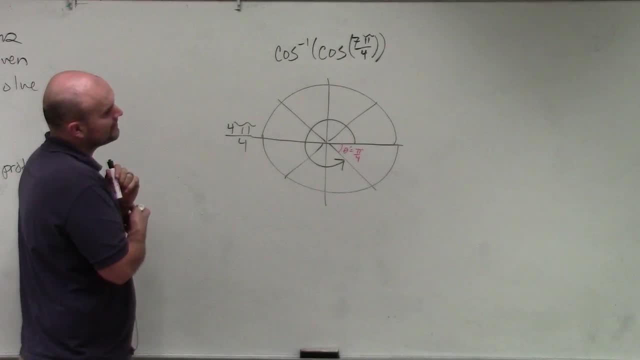 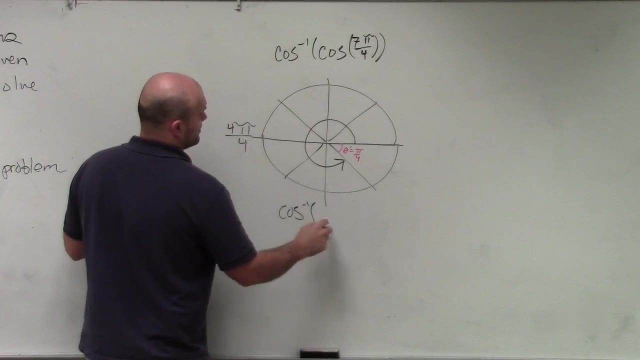 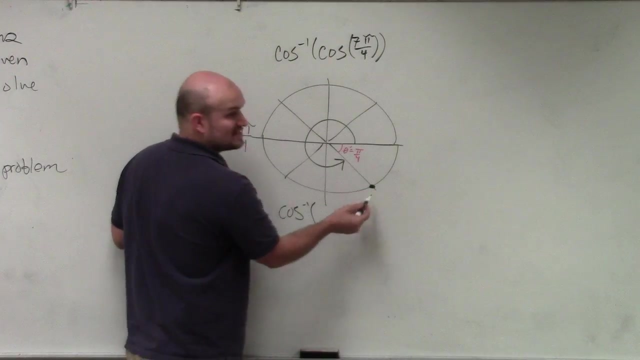 Square root of 2 over 2.. So, therefore, I now have the cosine inverse of square root of 2 over 2.. However, in this quadrant, though, is cosine positive or negative? So here's this point down here. So here's the reference angle, right. 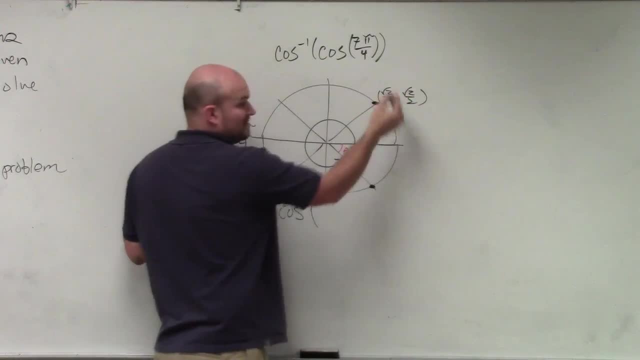 Square root of 2 over 2, comma. square root of 2 over 2.. Well, this point is going to be what's going to be negative? The sine right, The- oh, I'm sorry, the y-coordinate. 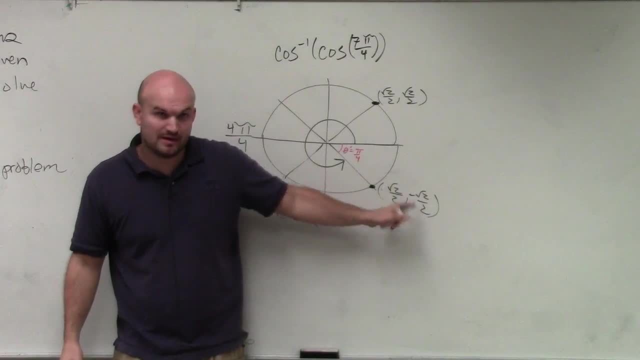 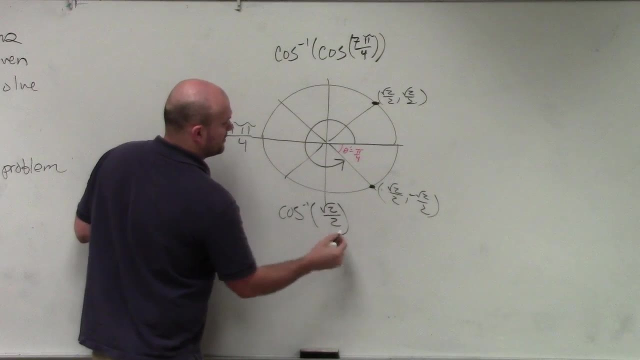 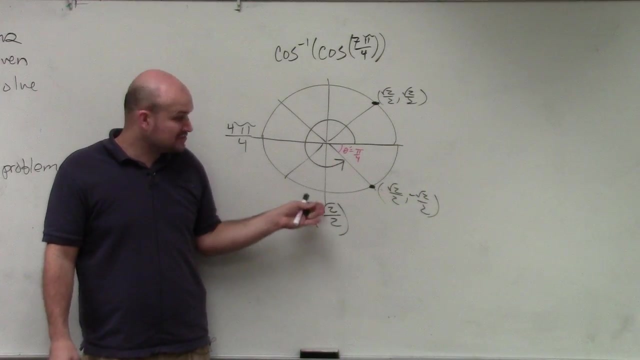 I don't know, But does everybody see how that one's negative Right? Only the y is negative, So cosine's still positive. So my angle now is cosine of square root of 2 over 2.. All right, So now I need to figure out what angle produces the positive value of square root of 2 over 2.. 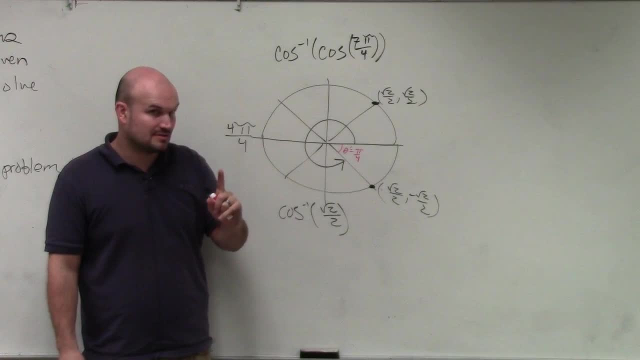 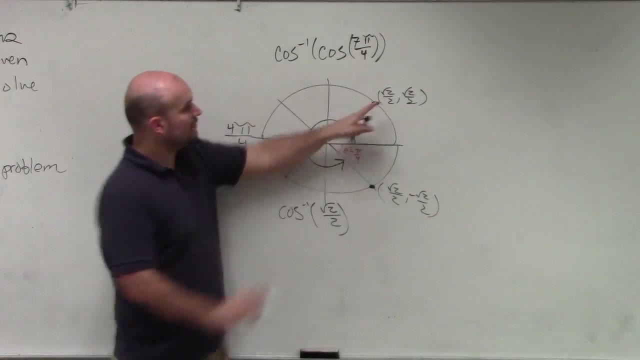 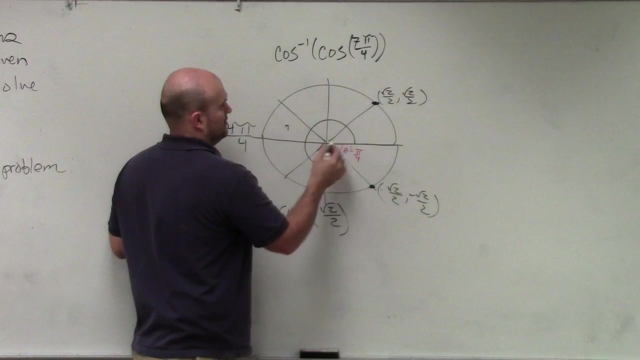 Well, there are Two angles. This produces the angle pi over 4.. Pi over 4 produces square root of 2 over 2.. And also doesn't 7 pi over 4?? This the original angle, the 7 pi over 4.. 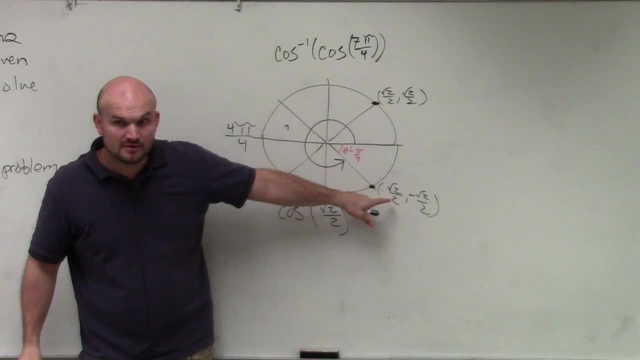 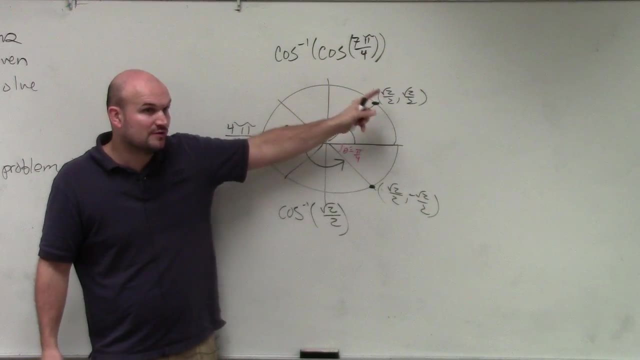 If you took the cosine of 7 pi over 4, isn't that also square root of 2 over 2?? Would you guys agree with me? So we have two answers. How do we know which one is correct? Because both of them produce square root of 2 over 2.. 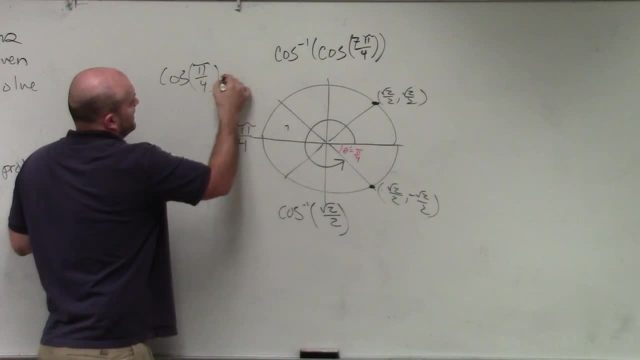 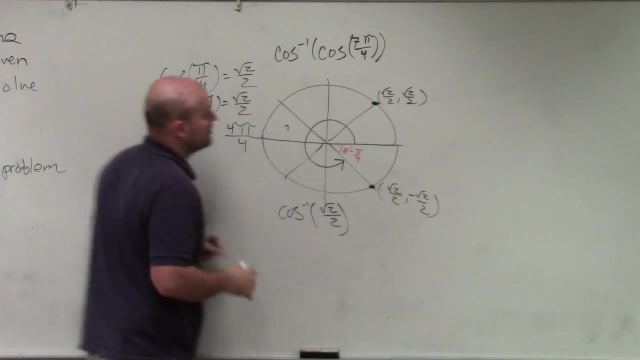 For instance, cosine of pi over 4 is square root of 2 over 2.. Cosine of 7 pi over 4 is also square root of 2 over 2.. So when I'm trying to say cosine inverse, I'm saying what angle produces the cosine of square root of 2 over 2?? 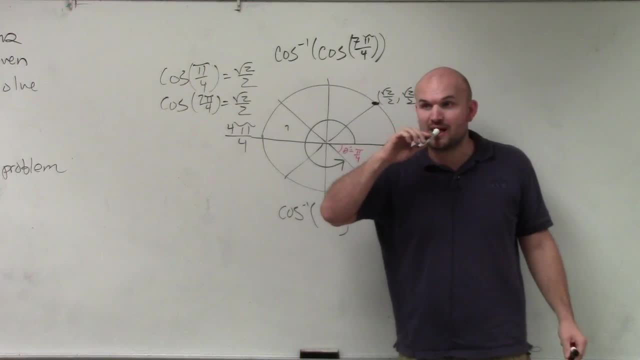 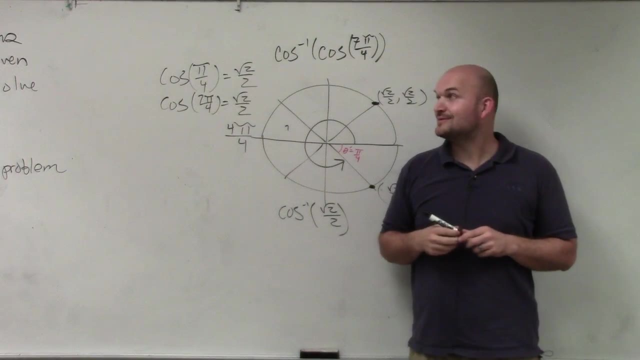 There's two options, but only one of them is correct. Yes, what do you think You don't know? Yes, Logan, Reference angle. Why I was like, will you always take the reference angle? It's always positive. 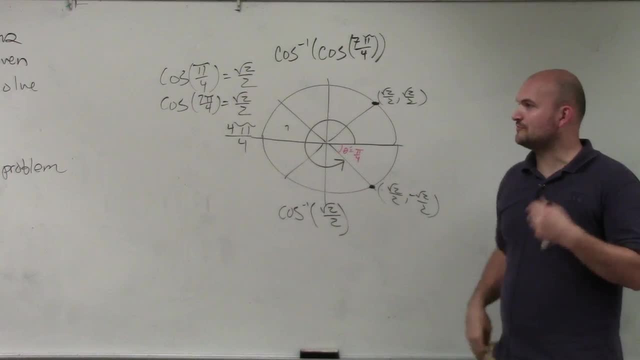 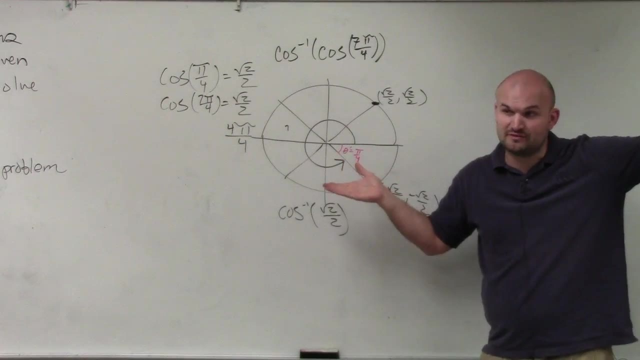 Well, I didn't really mean always use the reference angle for that reason, because it's positive- I always liked using the reference angle because it's much easier to remember, kind of like the points of the first quadrant. So if you can always remember what the reference angle is and then just evaluate for where it is in the quadrant. 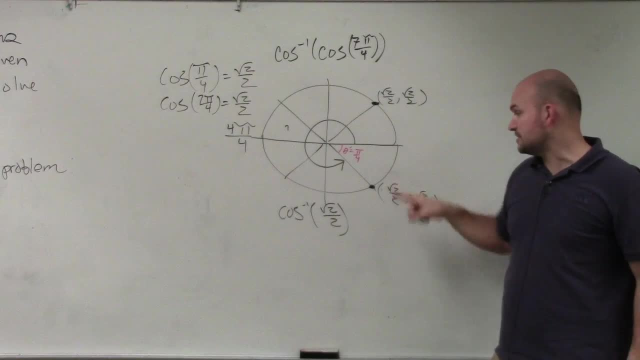 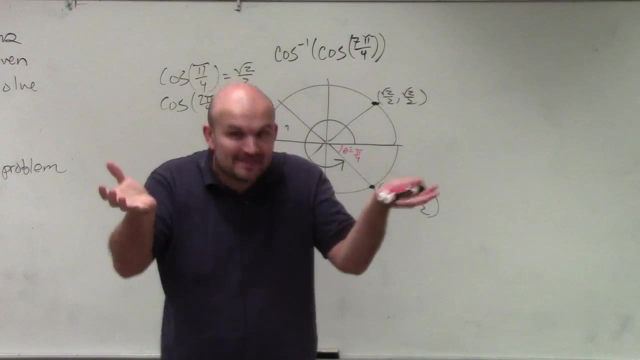 So if you know the reference angle, you know: oh, it's square root of 2 over 2.. Oh, it's in the fourth quadrant. That means that's negative, But there's an angle. There's one reason why the angle, and there's something that I spent 20 minutes explaining. 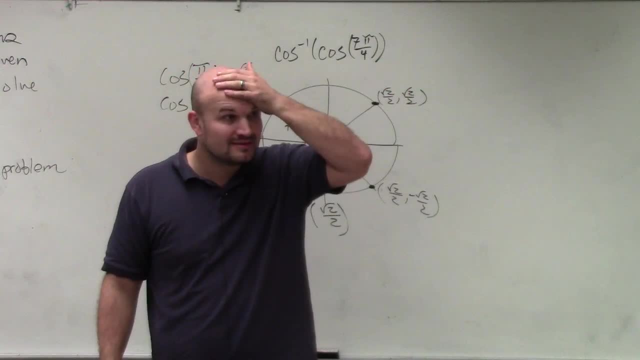 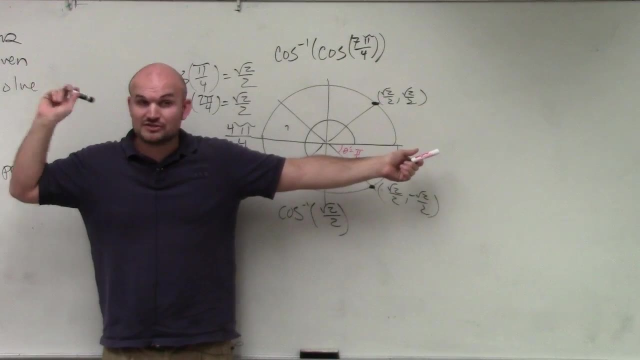 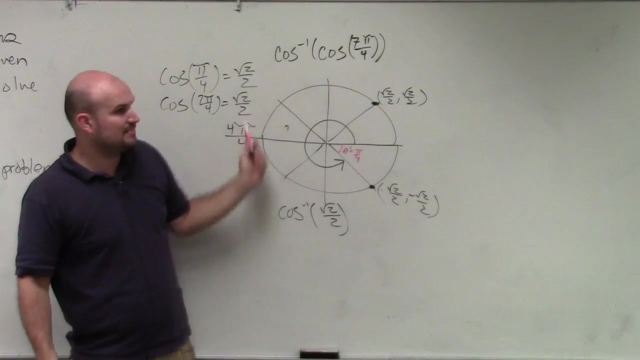 Explaining something about Because it's between 0 and pi. 0 and pi Because, remember I wrote down- you only have the inverse Sine. inverse is only a function when you restrict the domain of cosine between 0 and pi. 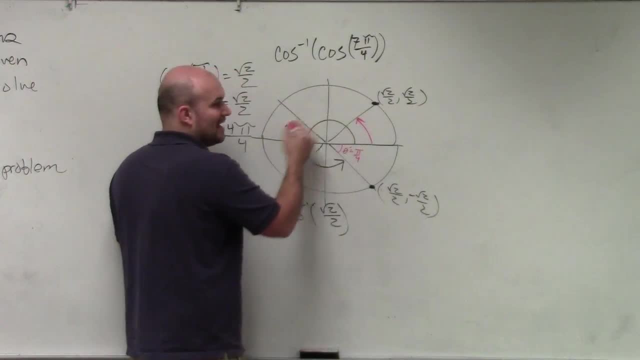 Do you guys see how this angle is between 0 and pi, Where this angle goes outside 0 and pi Yes. So therefore, your final answer is not: oh, they cancel, They cancel out 7,, 5, or 4.. 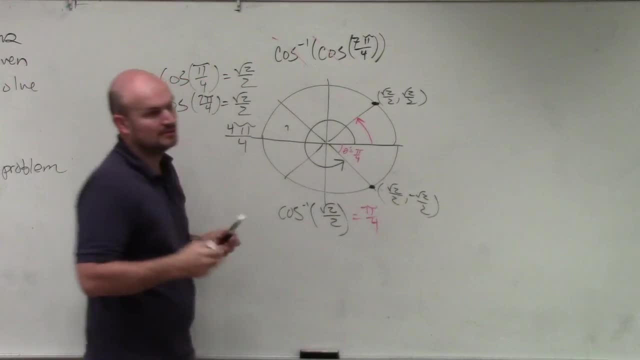 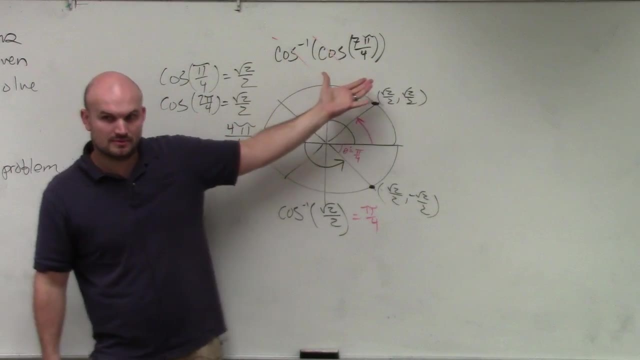 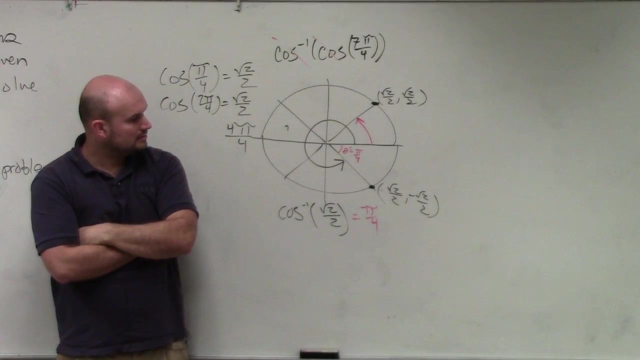 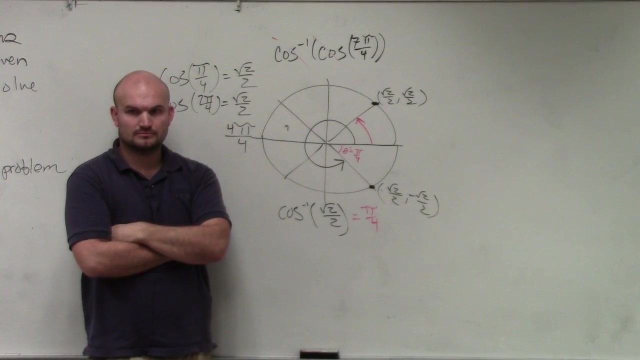 No, The answer is pi over 4.. Okay, So just from these problems. again, as I mentioned, do the innermost problem first, Then do the next problem. Okay, Yes, Yes, Pi, Yeah. Is that always circumstantial, with this being over that cosine? 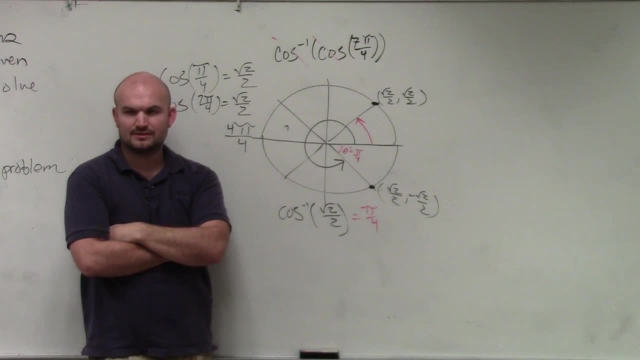 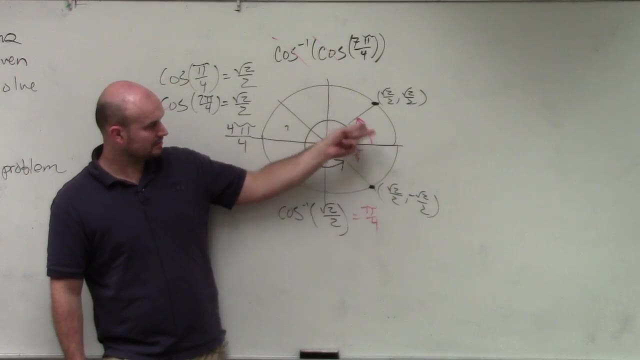 I'm not really sure what your question was asking. Okay, You found the last answer because this angle, the one that you have right now, The red one Right- Is between 0 and pi Right. The black one, The actual black one, yeah, 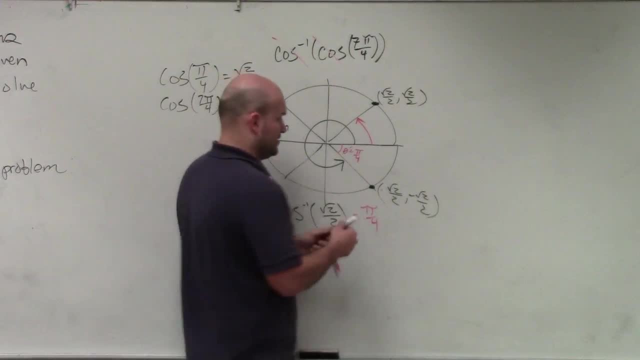 Which is 7 pi over 4.. Even though it produces the same x value, which would be cosine. do you guys see how they have the same x value Right? What do you mean circumstantial? What do you mean circumstantial?